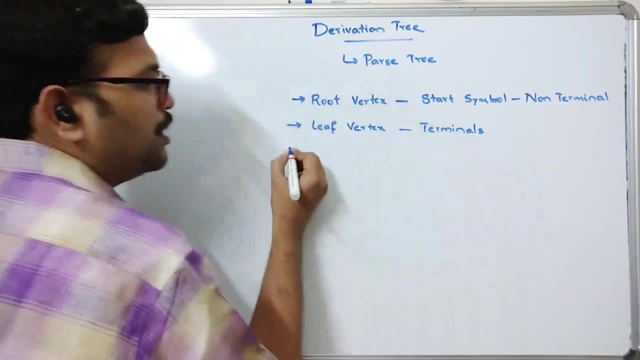 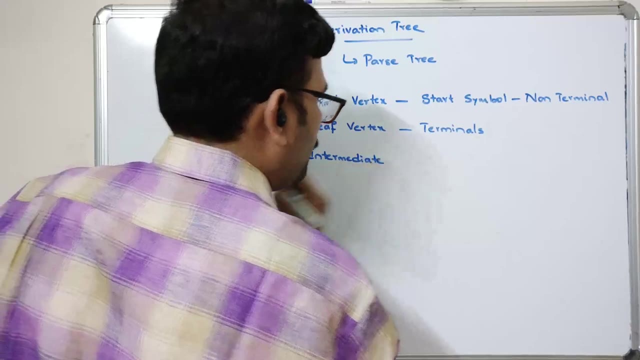 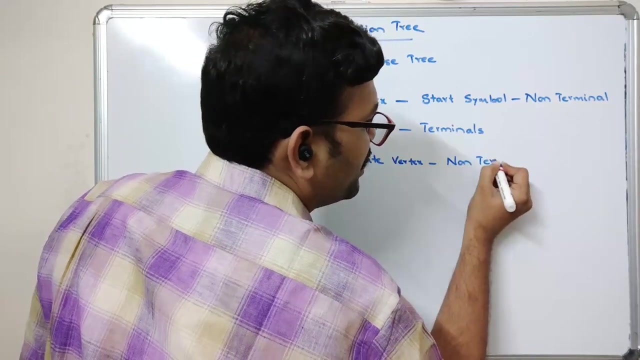 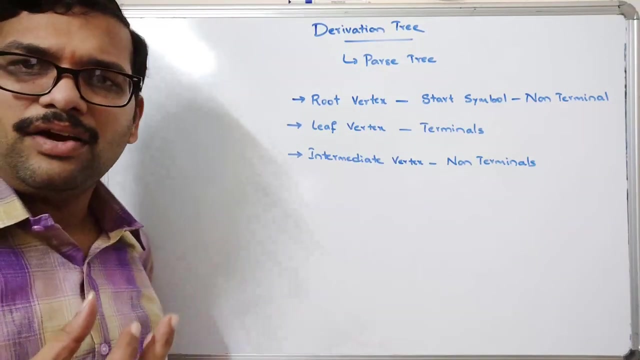 Terminals, Okay, And the third one is intermediate nodes, intermediate vertex. So these are all non-terminals, a set of non-terminals other than the start symbol. Okay, These are all the non-terminals. So if you consider any context-free, 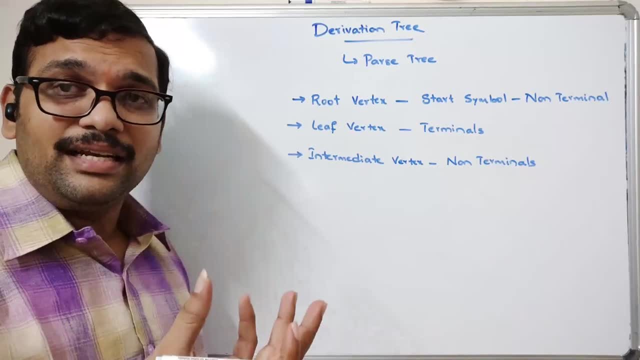 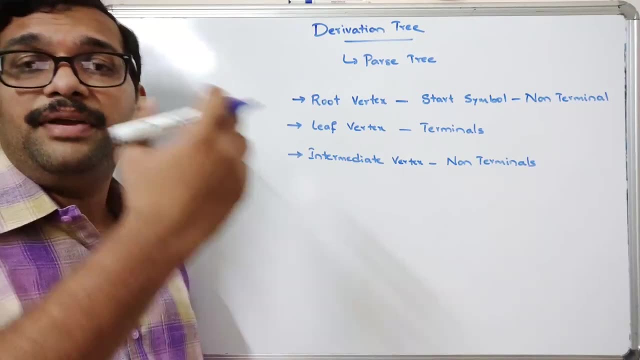 grammar. so is there any string which accepted by this context-free grammar can be derived by using some derivation, And that is a non-terminals. So if you consider any context-free grammar that can be graphically represented by using this derivation- tree Right, For example- 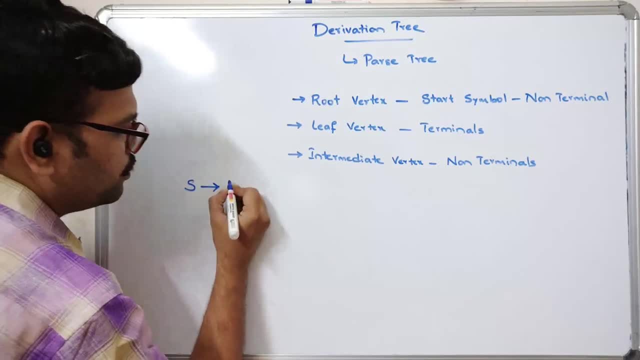 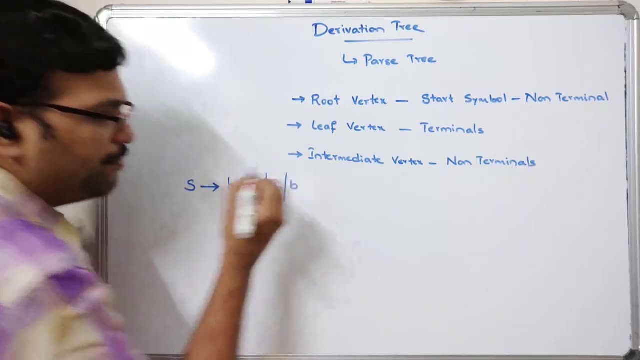 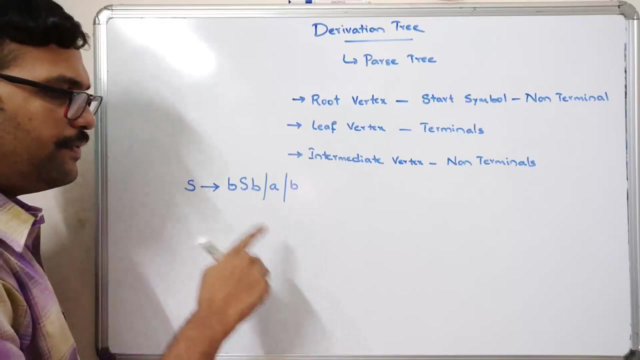 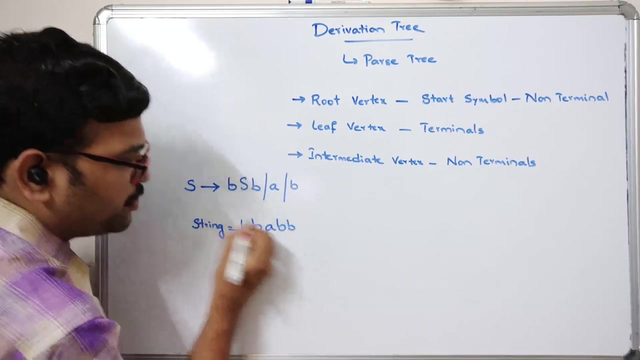 let us take some context-free grammar: X, S tends to some B, S, B or A or B. So let us take this example: Okay, And we need to construct the derivation tree for a string, for a string series A of B, A, B or A, B. So we need to construct the string So construction. 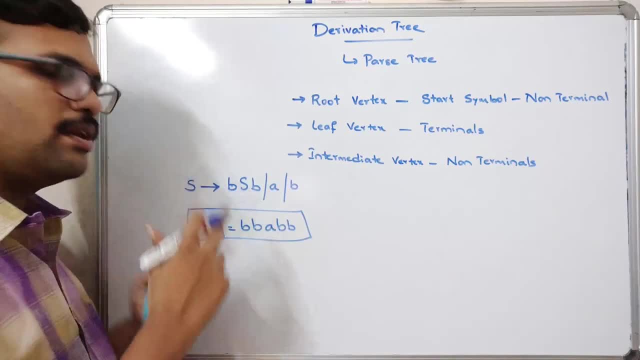 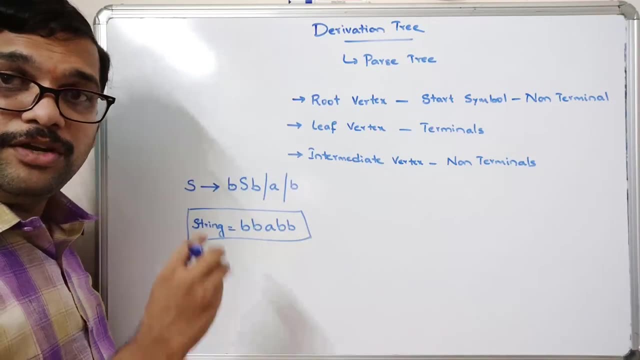 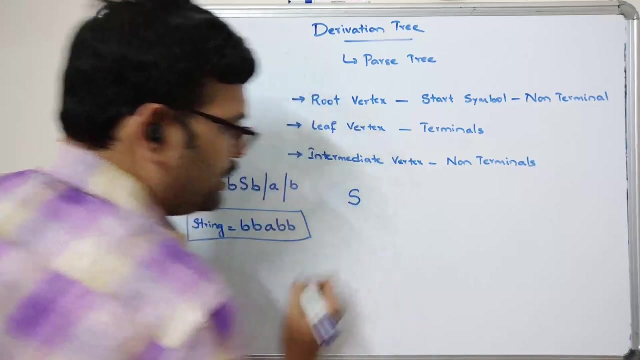 of a string means this string is accepted by this particular context-free grammar. So we need to derive the string from these production roots. Okay, We need to derive the string from these production roots, So let us start with the start symbol S. So in S we can substitute: 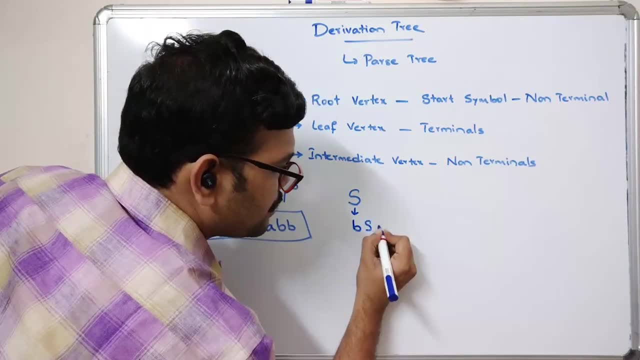 B S B. So B S B Okay. So we may actually ask, like, how many versus B S B? Now let's go ahead and come to B S B Okay. So B S B Okay. Let us remember that we need to. 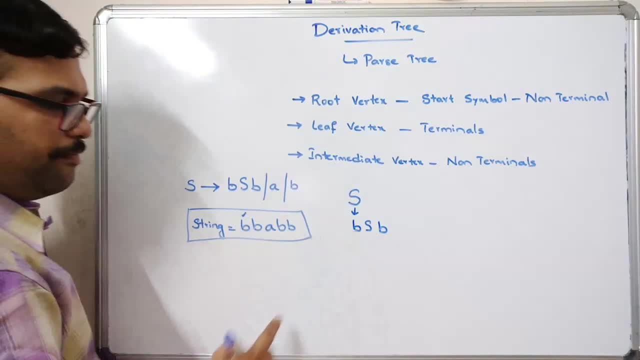 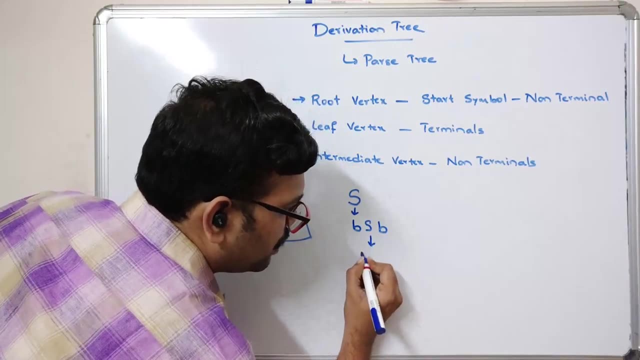 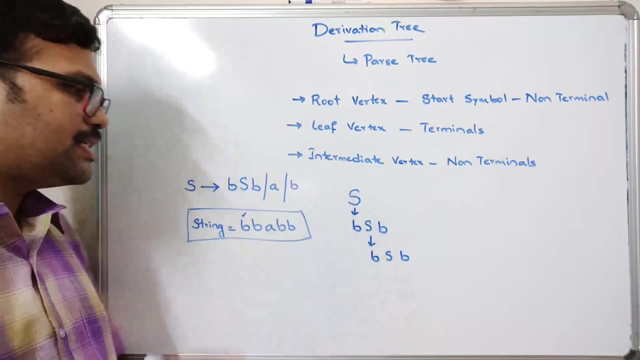 Okay, so the first B was done, and again S can be substituted with B S D. So again, once again, I will go with this one: B S D. Okay, so from the start. symbol: we are just substituting the production rules and deriving the string. 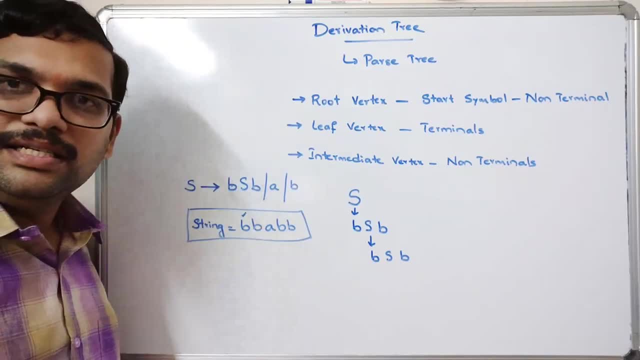 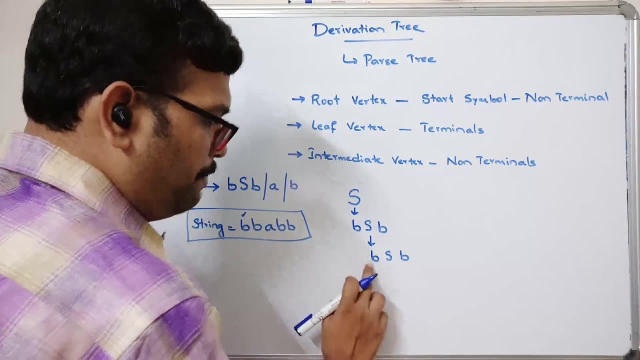 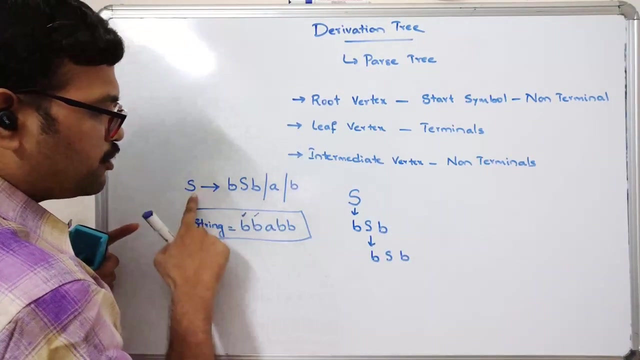 Because this string is accepted string by this particular CFG contextual grammar. So we are supposed to derive the string from this production rules. So you can observe here: B B, So this one also achieved B B. Okay, and also at the end we have achieved B B, Now A, So you can also substitute S with A. So if you substitute S with A, So you can observe here: 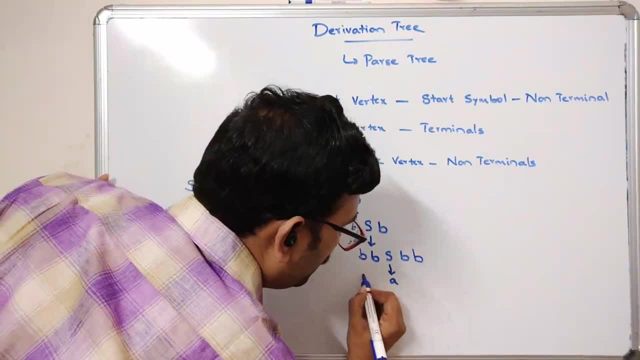 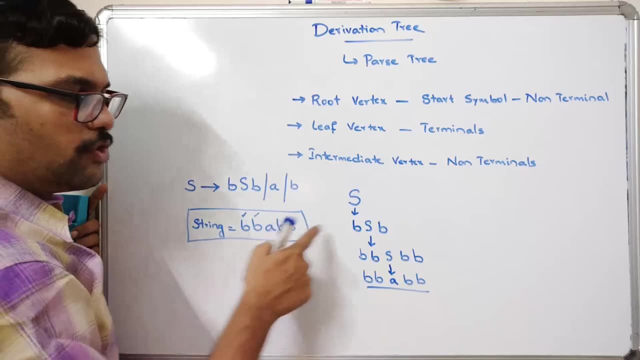 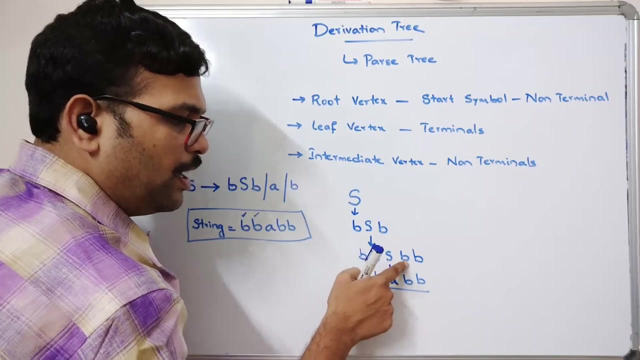 So it will be B and it will be B, and here you can observe B, B, B. So this is the required string. Okay, this is the required string. So, first of all, S is we have substituted B S B, and again in the S we are again substituting B S B, and in the S we are substituting S, so that we got this particular string. 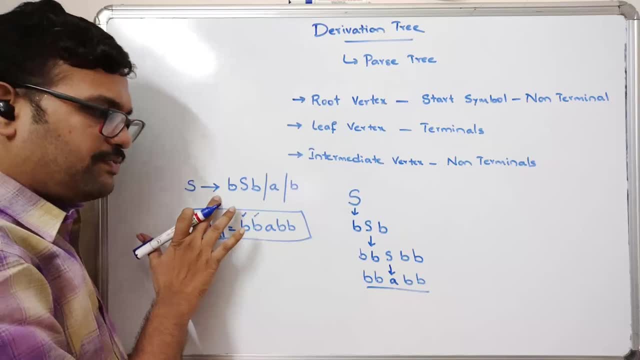 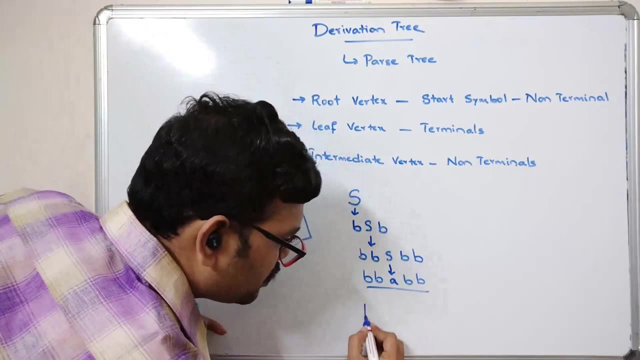 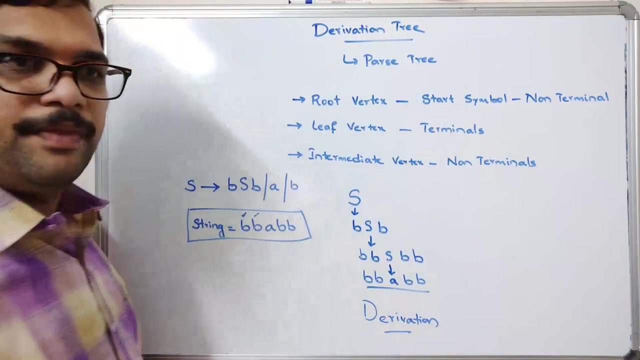 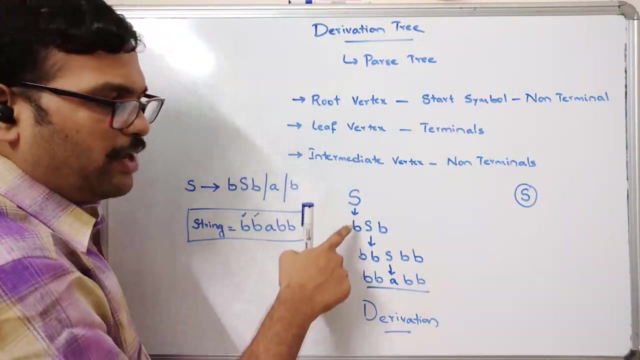 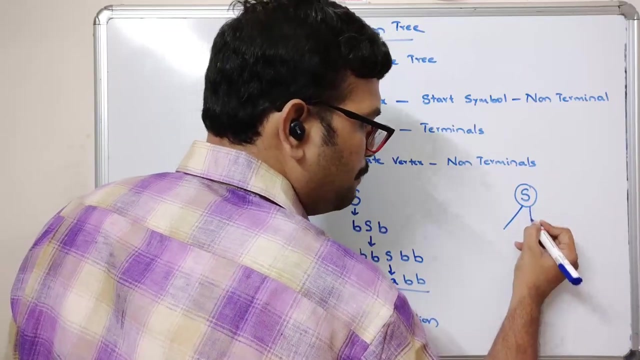 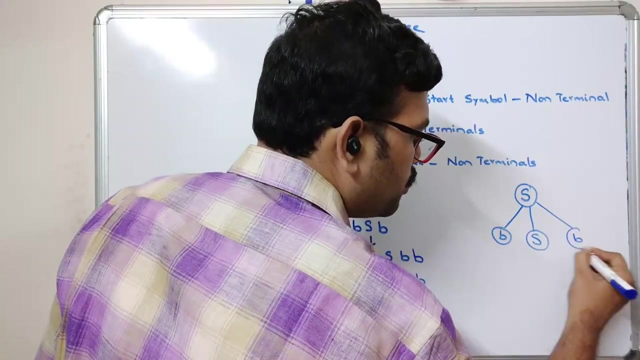 Right. So if the string is accepted by the contextual grammar, then we can derive that string by substituting the production rules and based upon this derivation. So this is called a derivation. Right, This is called the derivation. Okay, And from this derivation we can easily construct this derivation. So what is the start symbol? root vertex. That is a start. Yes, Right, This is the start symbol. And S by S we are substituting the another production, that is S B S B. So it will be having the branches B S B. So this is a B S B. So here you can observe, B are nothing but a terminals. 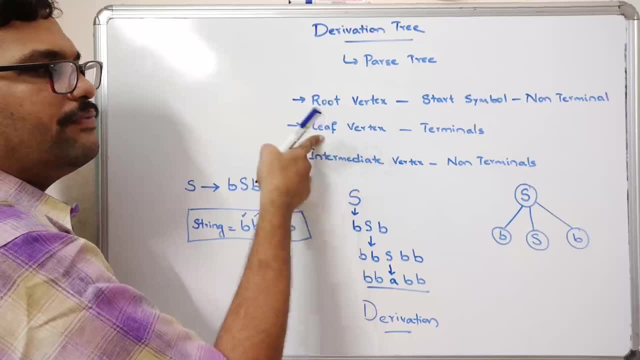 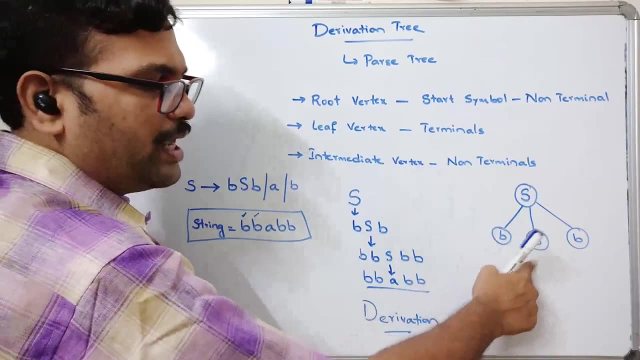 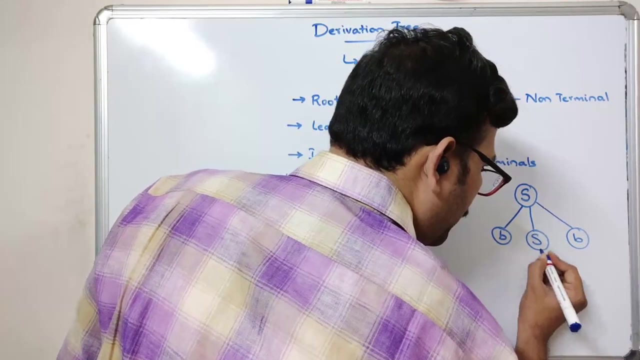 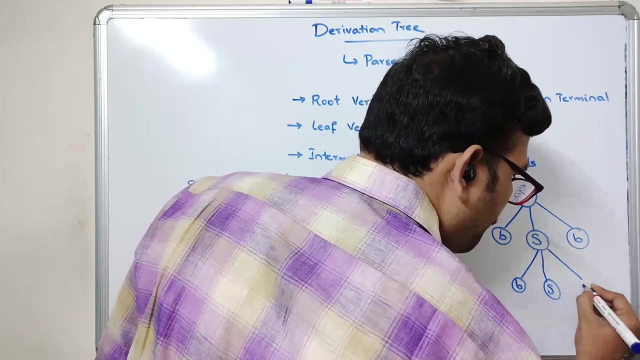 Yes, Yes, Yes, Yes, Yes. a terminal. automatically it will be the live vertex, so there will be no expansion right, there will be no branches and s is a non-terminal, so it is a intermediate, so we can expand s again, right again, in order to get the given string, s should be again divided into b s, b, b s b. 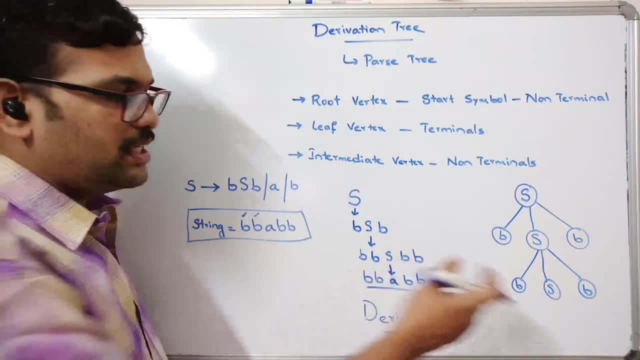 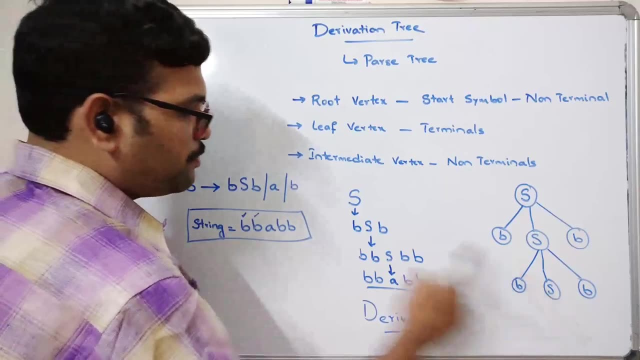 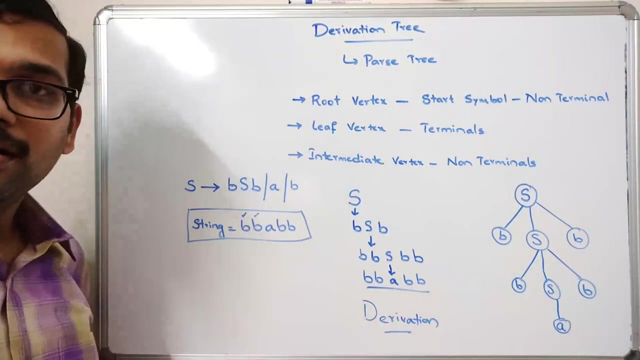 so again you can observe: b are the terminals we can't expand, so these are the live nodes. now again we can substitute s. so in order to get the given string, s should be substituted with a. right now i will expand this one with a. now you can observe: a is again this terminal, so we can't expand it. 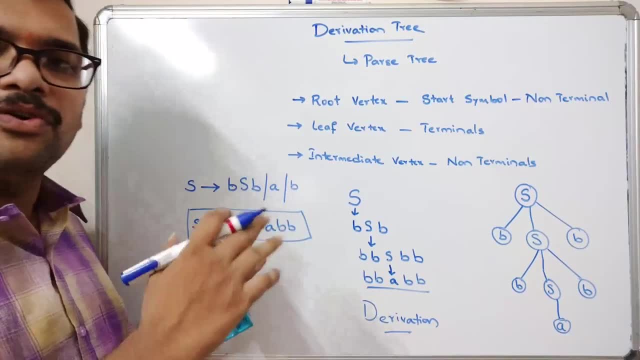 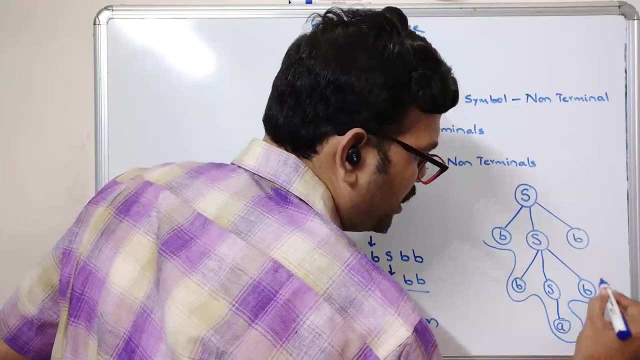 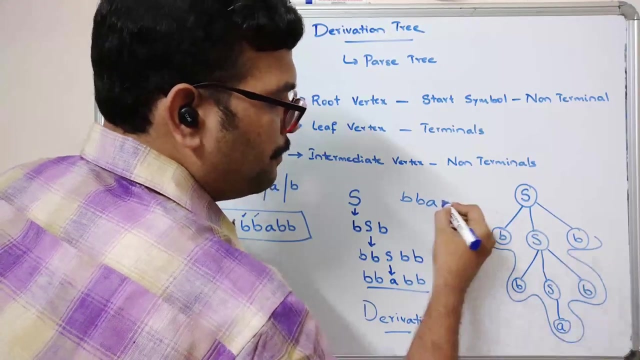 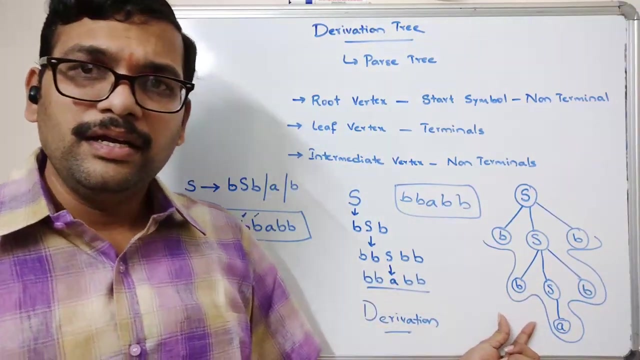 now just read the live nodes from left to right so you can observe here: so b, b, a, b, b right. so b, b, a, b and b. so this is the string. you got this string right. so in order to draw the derivation tree, so it would be very easy if you derive the string from the production rules. so 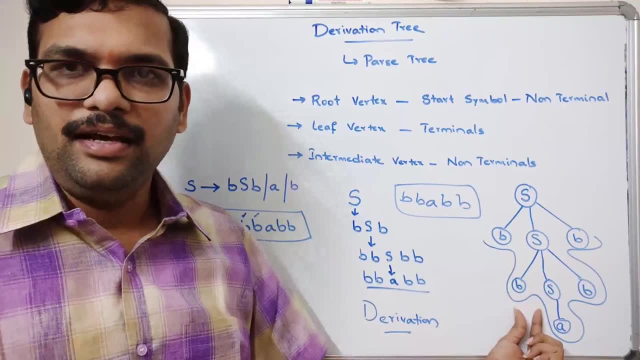 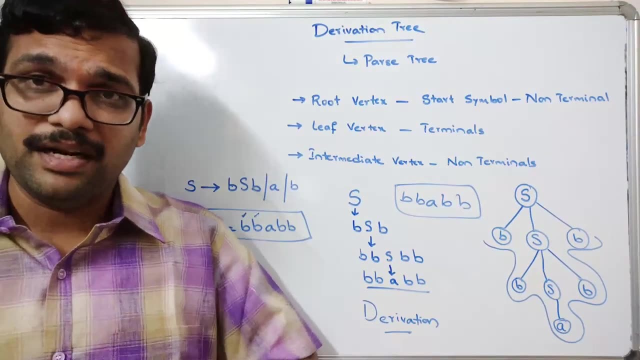 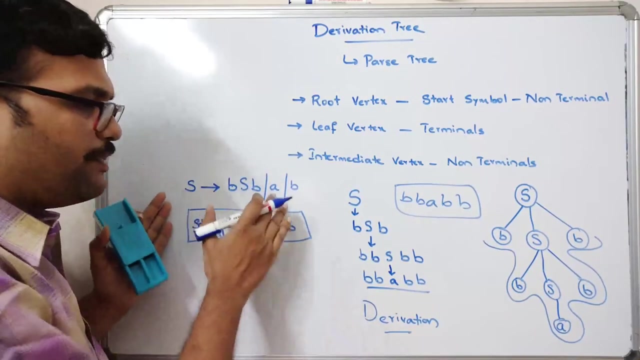 from this derivation so we can simply write the derivation right. so hope you understood. first we need to take the string which is accepted by the contextual grammar and we can directly so here the strings that accept by this contextual grammars will be many. so, for example, if the string is b, a, b, this is also. 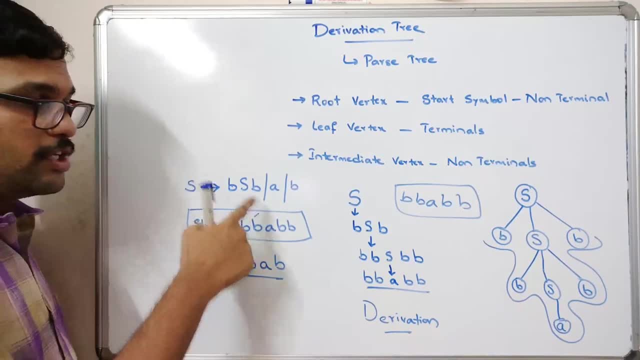 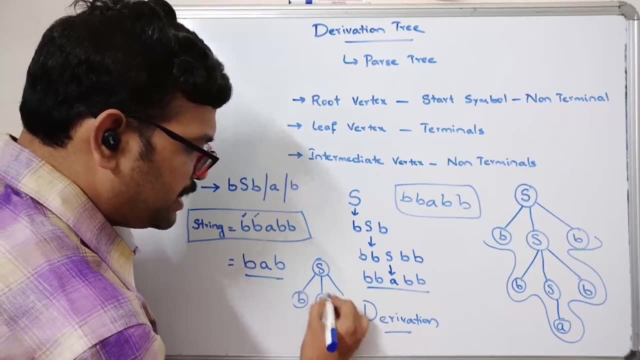 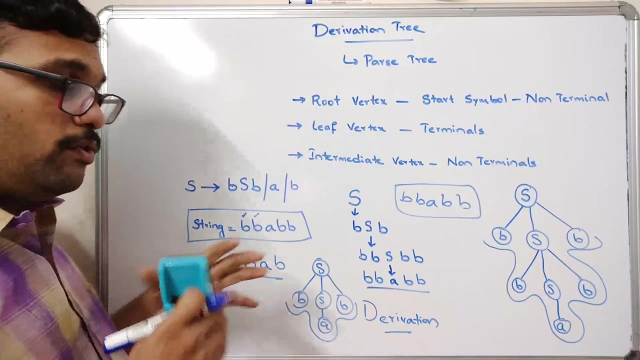 accepted string. this is also accepted string, right. so we can also draw the derivation tree for this one. so b s, b, and here it will be a. so you can observe here: b, a, b right. so we need to read the leaf nodes from left to right in order to get the string. so here we. 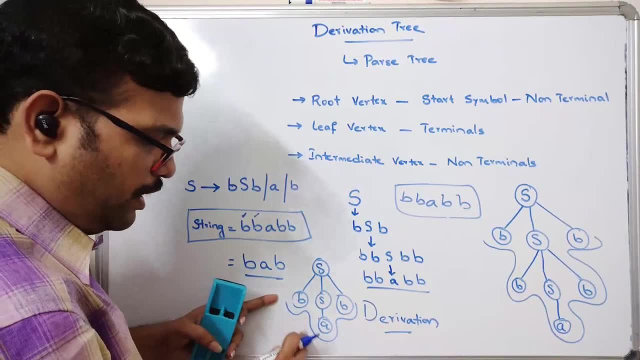 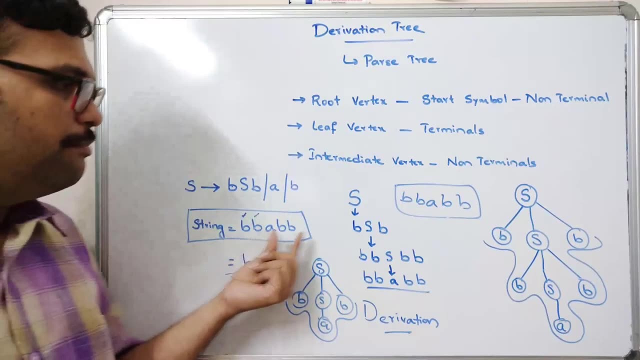 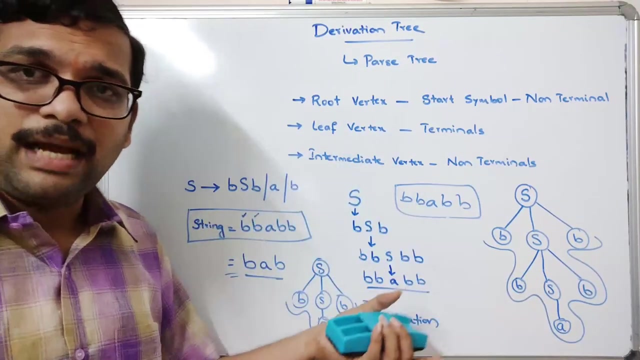 are reading from left to right, so from leftmost, so b a b. so this is s, s, so b a. so we can consider any string and just derive that string by applying the productions and directly from that deviation we can simply draw the derivation tree. so we will see one more example for this derivation tree, which nut for this derivation tree compensate. so we will see one more example for this derivation tree: how deselect right? so consider the one more example. supposing that this is the了吧 right, we could just just give it our hint: define when is that going to be defined? and we do not, because we keep. 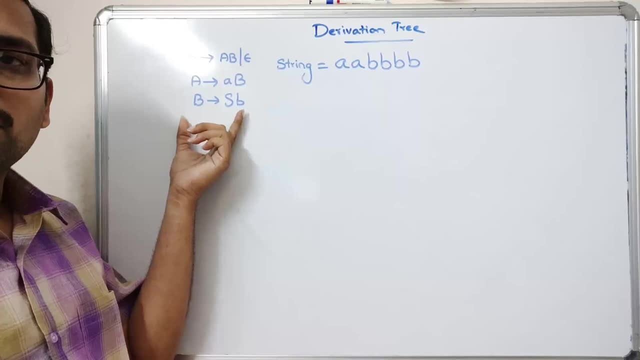 note this: one more session. we are going to reduce the totally we went out. this, you know, limited by certain that haven't limit. what should is from this you can just find the Golf and gorilla from this certain on the course. this is the production rules, right? So this is the conductive grammar. So S tends to AB or 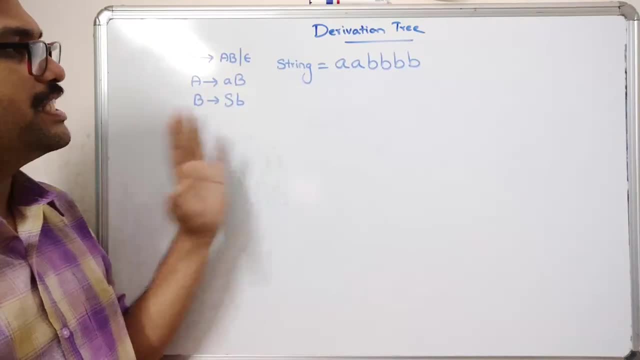 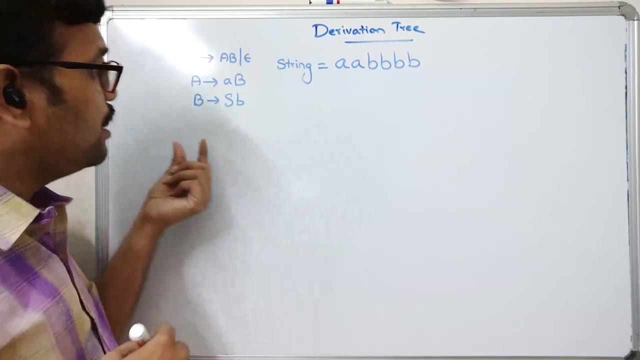 epsilon A tends to AB and B tends to SB, and the string is here. So we need to construct the derivation tree for this one. So before constructing the derivation tree, first let us derive the string from the production rules. So I will write this one above. 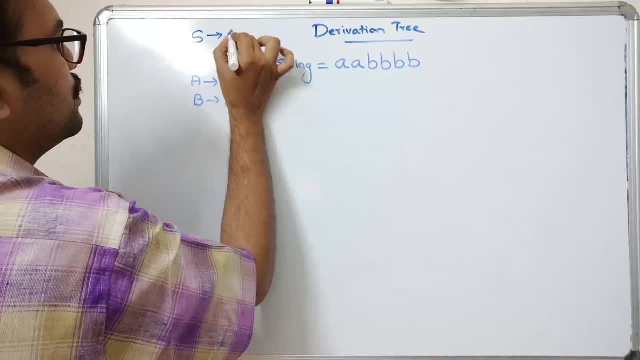 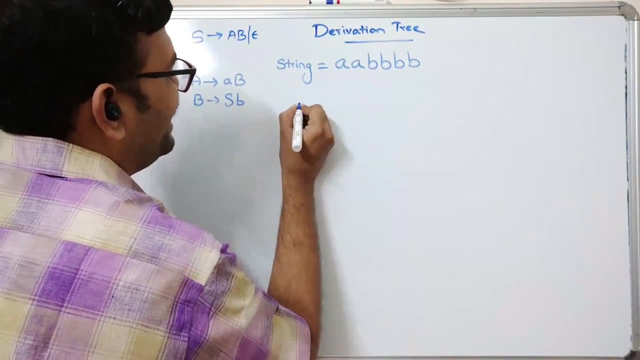 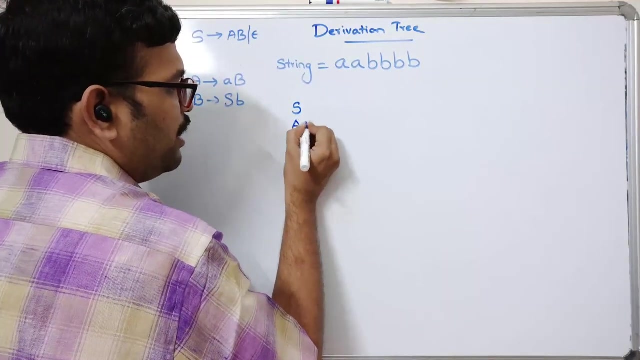 I think it is visible. yes, So AB or epsilon. right Now, let me start with S. So S can be substituted with AB or epsilon. So I will just write AB. and now. first we need to get the terminal A, So in order to 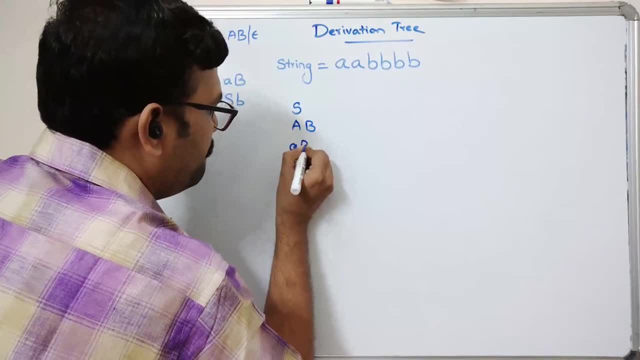 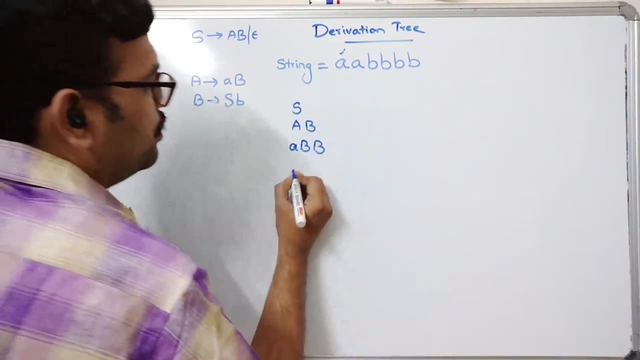 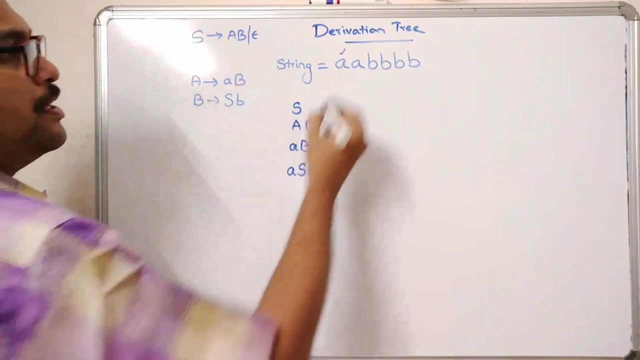 get the terminal so A can be derived as ABB right. This was achieved and again we need to get A. So in order to get A here, you just write S, B and B. So now this A is sorry. S A, A, S B. 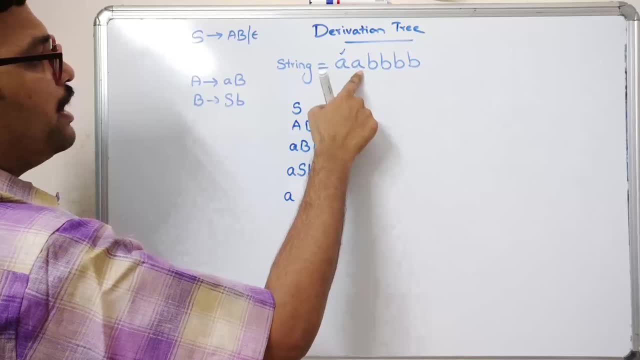 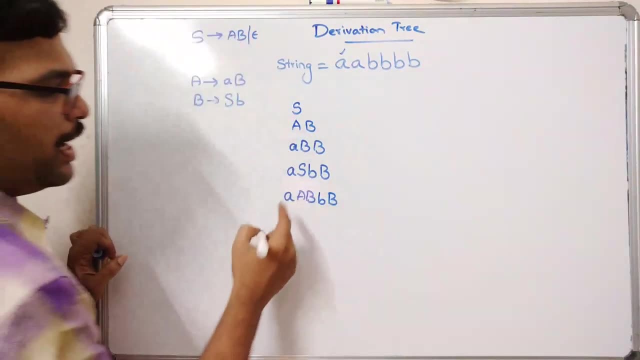 right And again. so if you want to get A, just we need to apply S as A, B, B, B, And again, now instead of A. so we need to get this one right. So A instead of. 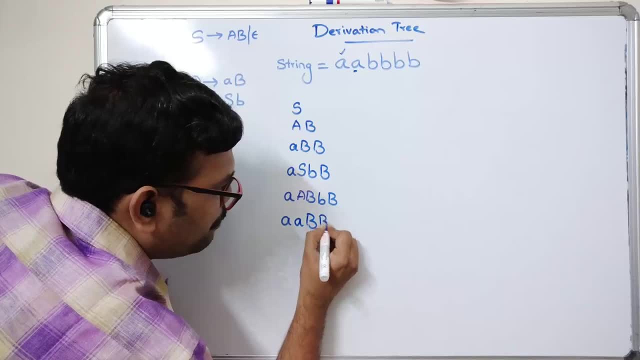 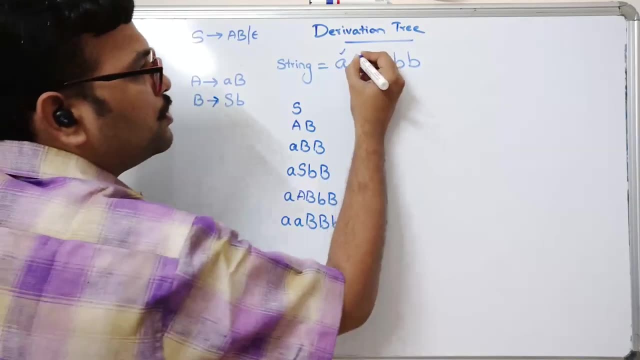 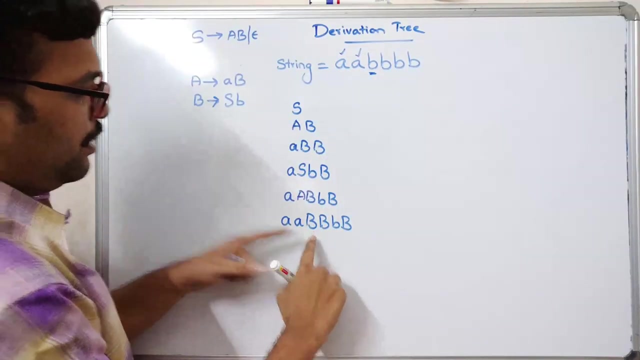 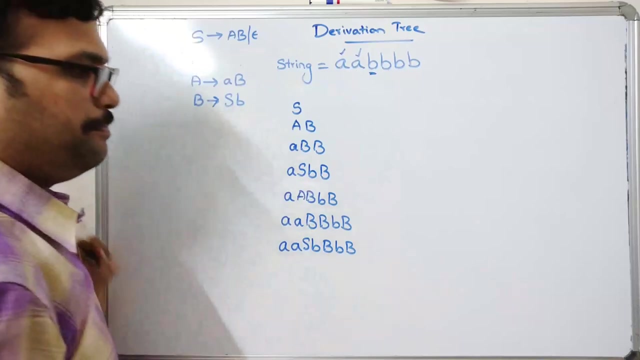 A. we can write ABB, B, B and B. right Now you can observe here two S's have been achieved. Now we need to get a, B. So instead of B here you can write it SB, B, be and B. 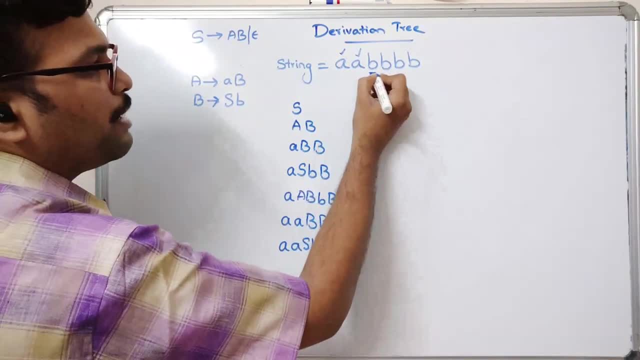 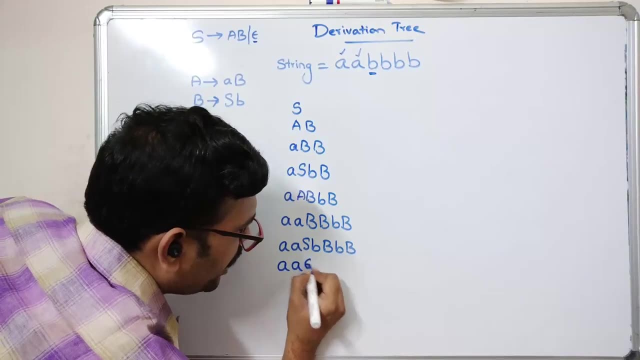 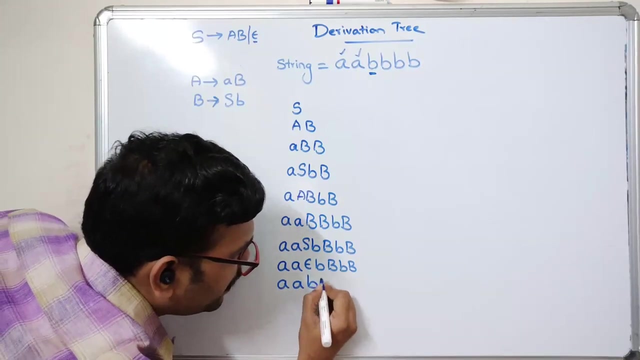 okay, Yes, So you can observe, here We have to get a- B. So instead of S we can simply apply epsilon. So this will be A A, epsilon B, B, B and a- B. So you can simply avoid the epsilon A A, B, capital B, small b and a capital B, And again. 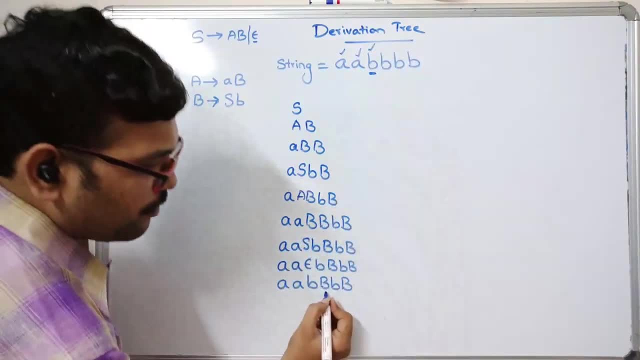 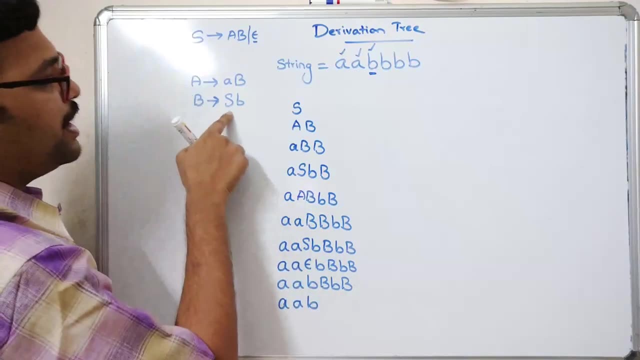 so this was H E. Now again, we need to get a B here. So instead of getting if you are forgetting B now again, substitute this one: A, A, B and B can be written as S B. Again, you can write S B. 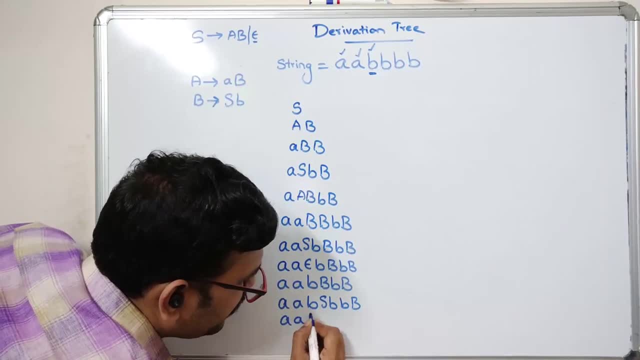 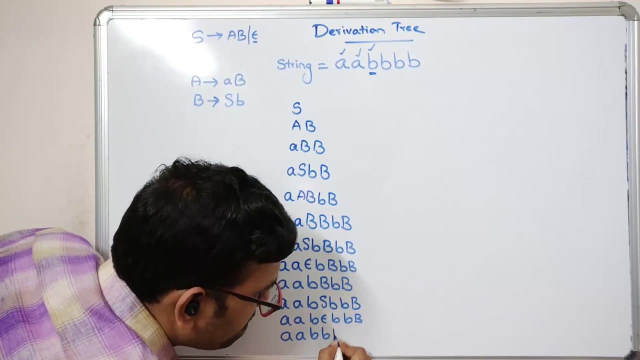 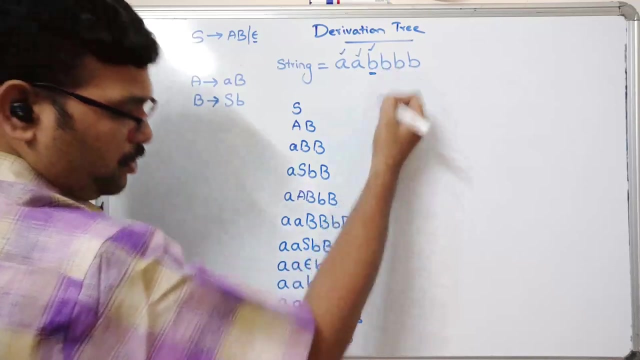 B and a, B. Again you can apply the epsilon A, A, B, epsilon B, B and B. So avoid the epsilon A, A, B, B, B and B Again. you need to expand this B. So we have achieved this one Up to here. we. 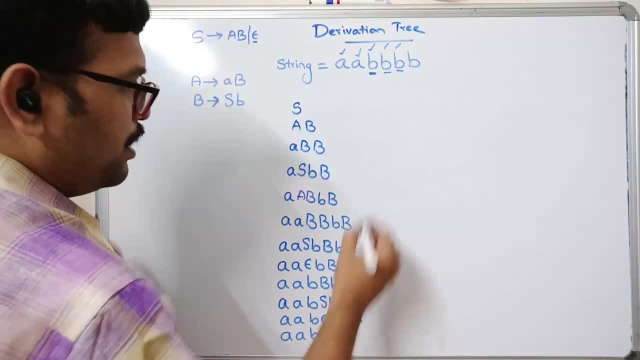 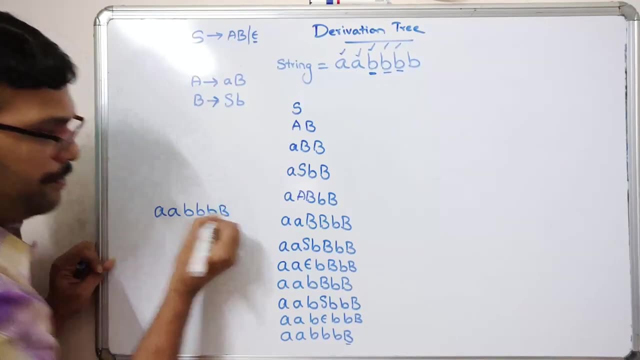 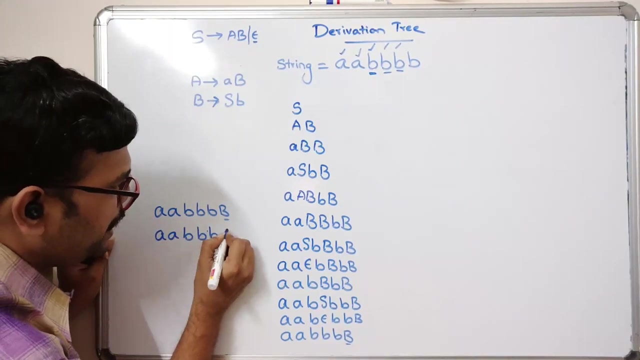 have done right last B, So this will be done. I will write here: So: A, A, B, B, B and a, B, right. So instead of B again, I am just substituting here A, A, B, B, B S. Sorry, this is B S, Sorry S, B, okay S. 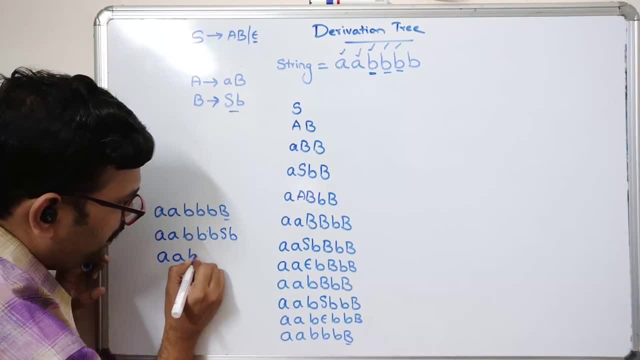 B. So right Now, A A, B, B, B. epsilon B. So simply we can avoid the epsilon A, A, B, B, B and B. So this will be done. I will write here. So A A, B, B S. Sorry, this is B S, B. So 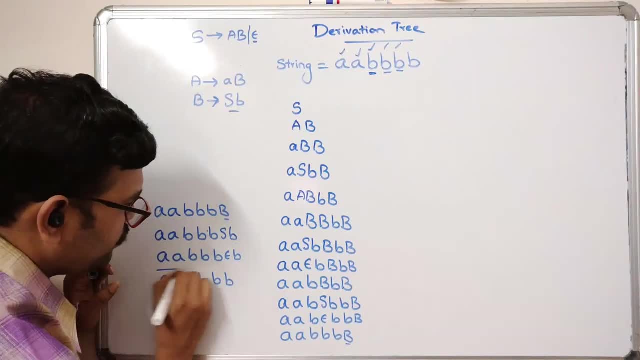 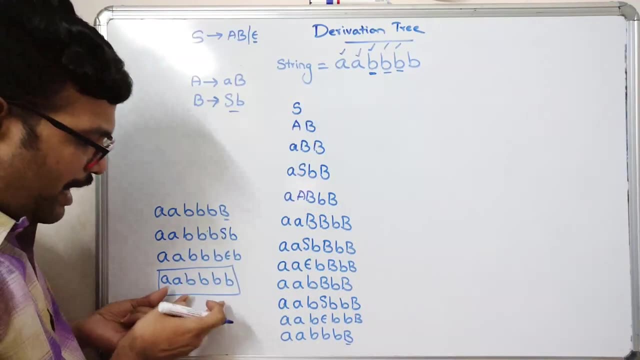 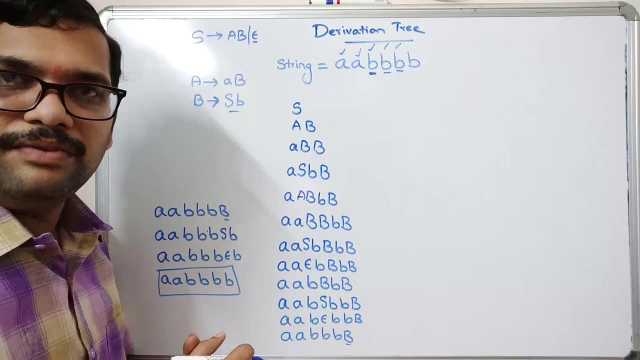 avoid the epsilon. so simply, we will get this one. so this is the string. so this string was derived from the start symbol. okay, simply, we are deriving the string from the start symbol. so just represent the same derivation using the derivation tree. so start with symbol s. start with symbol s, okay, 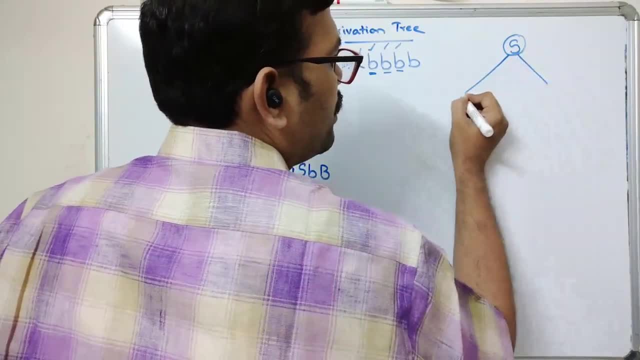 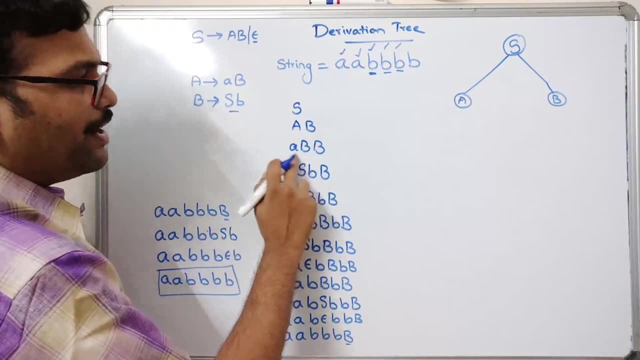 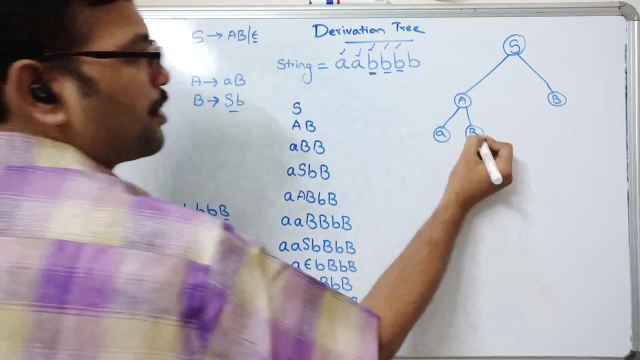 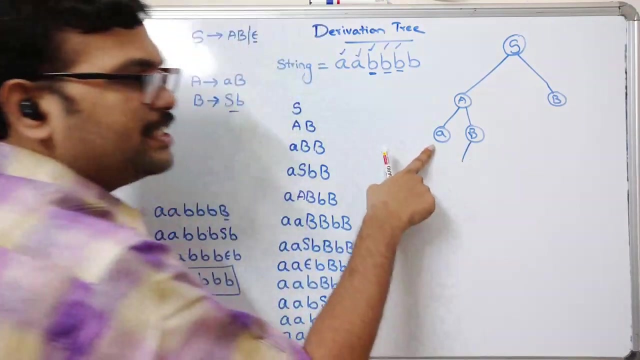 so yes, first we have given a and b. next step: a is again divided into ab, so a, b, right, and again b is divided into s, into b, so so we need not change this one because this is a right, so s and b. so we need not change this one because this is a terminal right, so s and b. 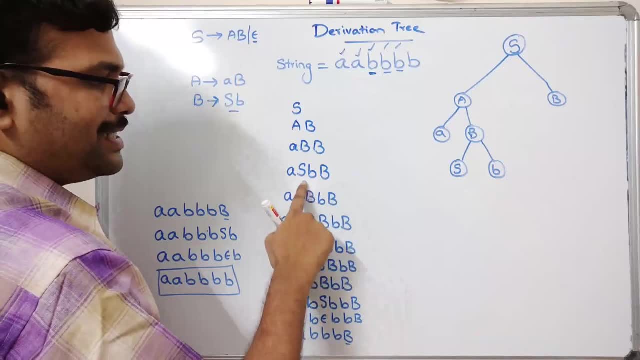 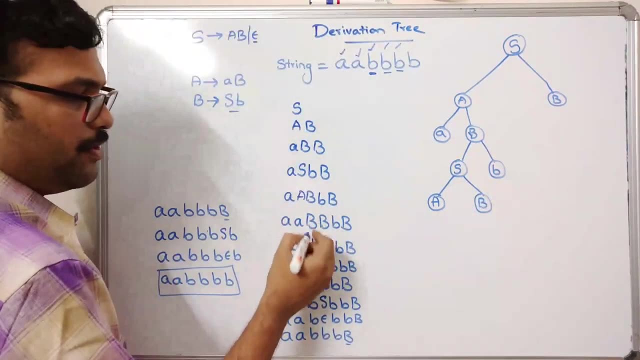 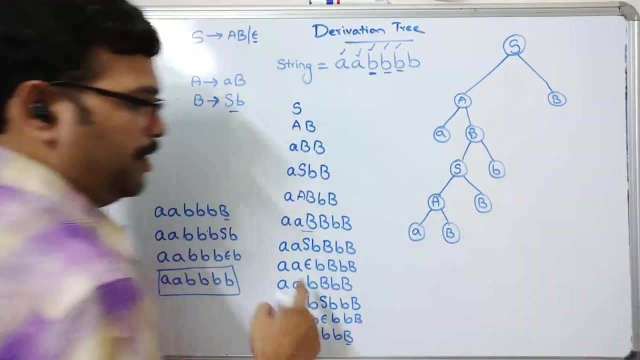 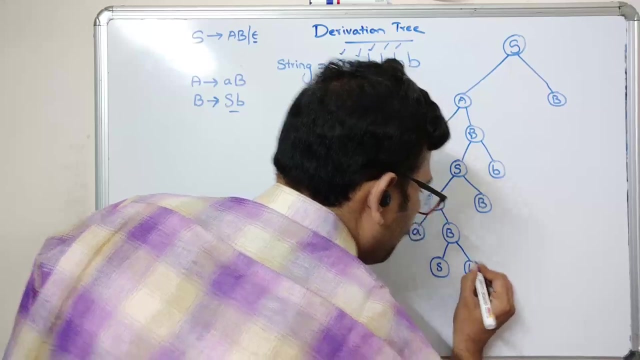 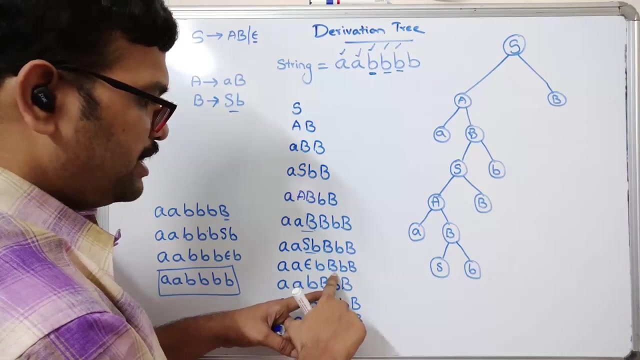 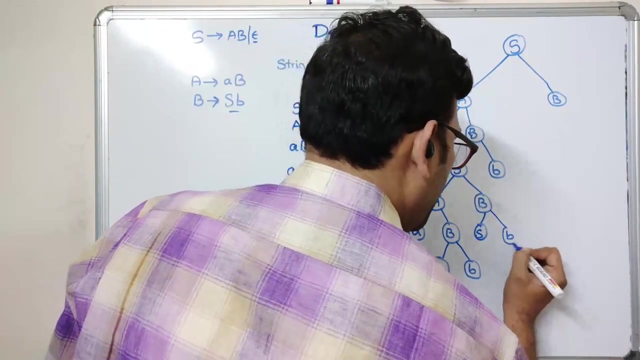 right, we have to change b again. this s is divided as a, b. so once again, a, b, okay. and again a is divided as a, b, a, b, okay. now again b is divided as s, b, yes, b, right. and now c, this b is again divided as yes, b, yes and b. and here, uh, we have given some epsilon, we have given. 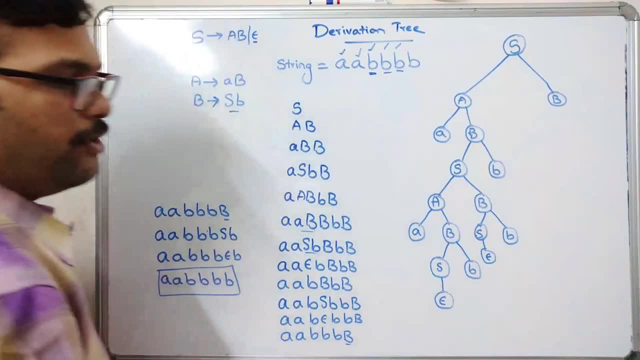 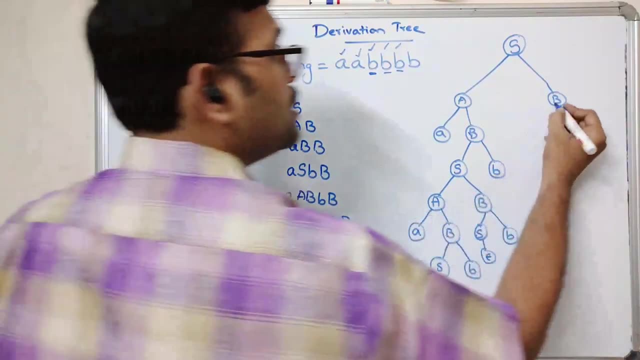 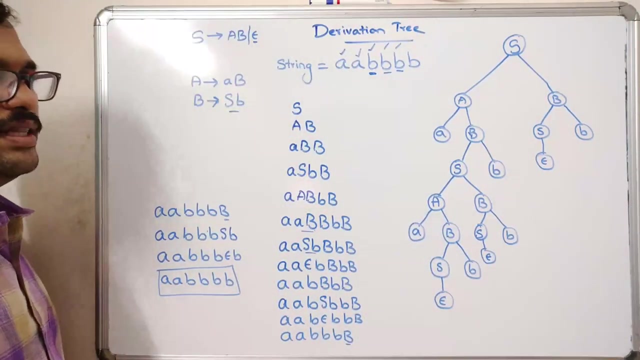 some epsilon, and here also we are giving some epsilon and you can see a, a, b, b, b, and here again b is divided as yes and b, which is nothing but epsilon here. so this is the right one, so this is the left one. so this is the right one. so this is the derivation tree. 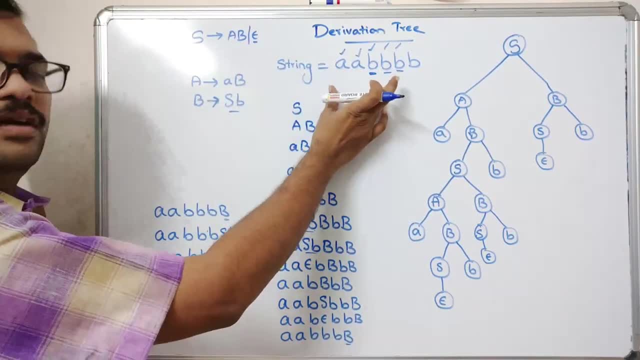 derivation tree: for this particular context, with the amber, to achieve the. for this particular context, with the amber, to achieve the. for this particular context, with the amber, to achieve the string, string, string for two years, followed by four weeks, so you for two years, followed by four weeks, so you. 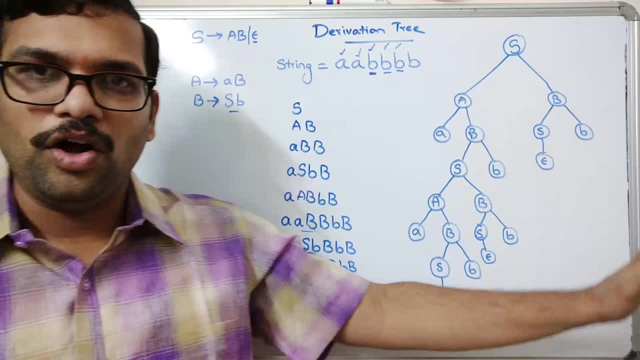 for two years, followed by four weeks. so you have to read the string from left, to have to read the string from left. to have to read the string from left to, to write all the leaf nodes from left to. to write all the leaf nodes from left to. 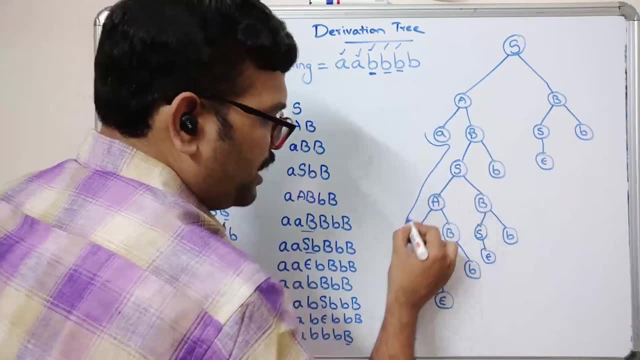 to write all the leaf nodes from left to: to write, to write. to write: see a. and what is the next one? a see a. and what is the next one? a see a. and what is the next one? a. what is the next one? epsilon b b. what is the next one? epsilon b b. 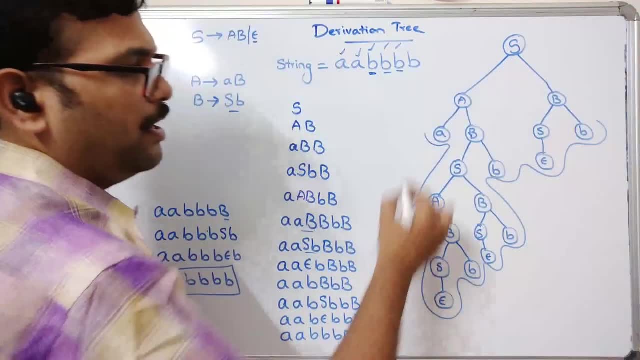 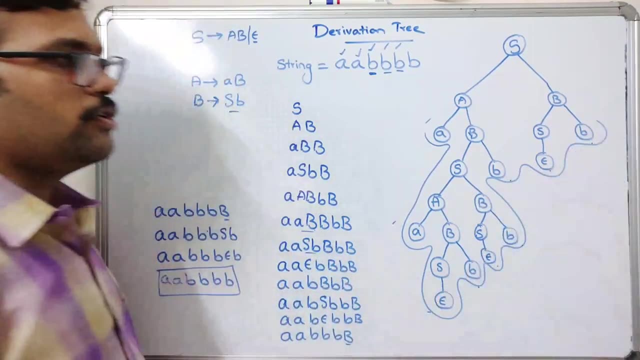 B- epsilon B right. So A A- epsilon B, epsilon B- B epsilon B. So from reading from left to right we are achieving this particular string. So this process we call. 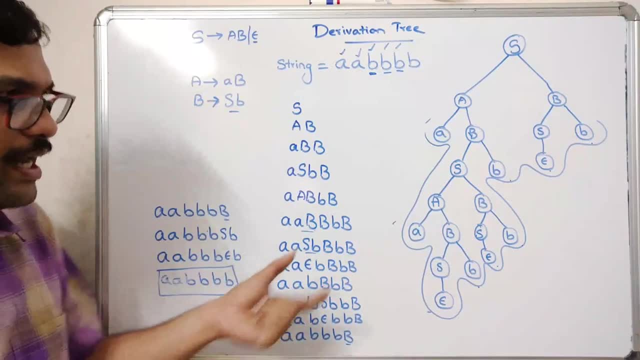 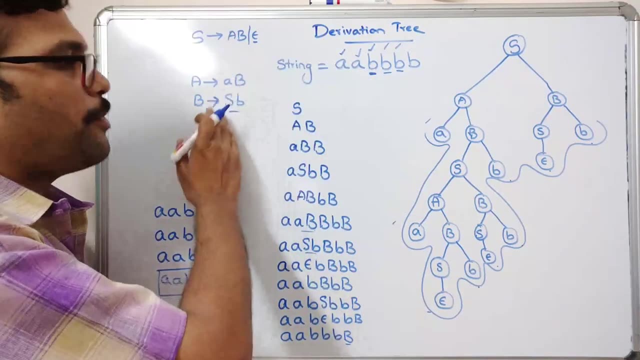 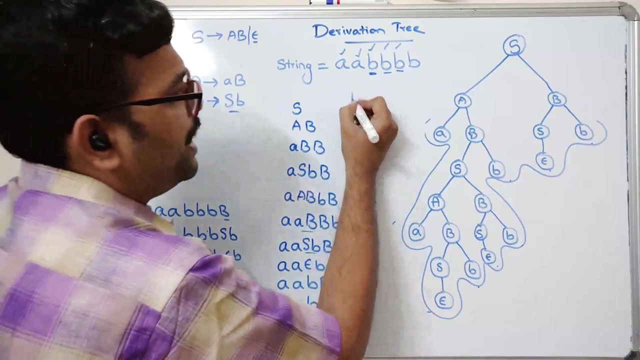 it as a derivation tree. So this is called a derivation and this is the derivation tree. So if you derive this, if you derive the string from the production rules, then it will be very easy to draw the derivation tree. and this derivation tree is also known as parse tree. 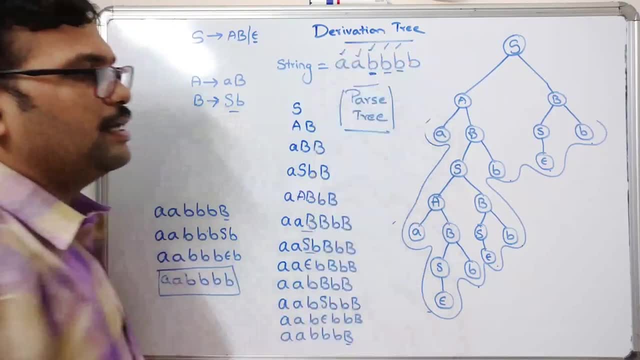 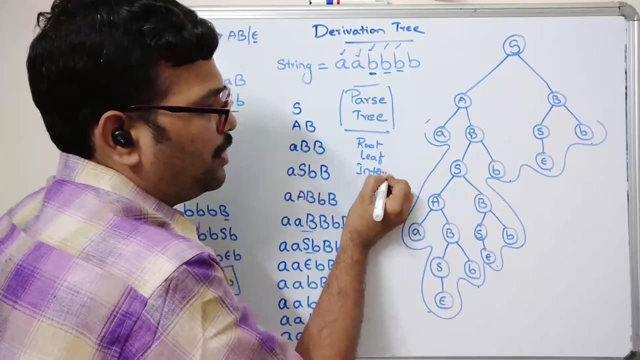 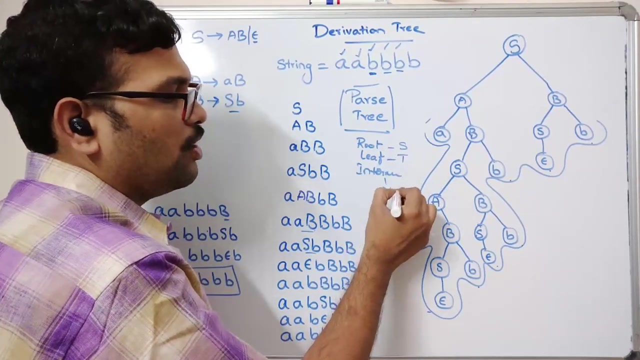 Parse tree- okay, derivation tree- or a parse tree. So three nodes will be there. One is a root node, another one is a leaf node, another one is a intermediate node, intermediate node. So root node is a start symbol, leaf nodes are terminals and intermediate nodes are non-terminals. 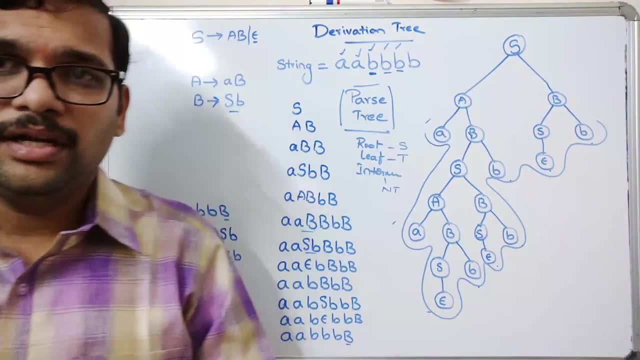 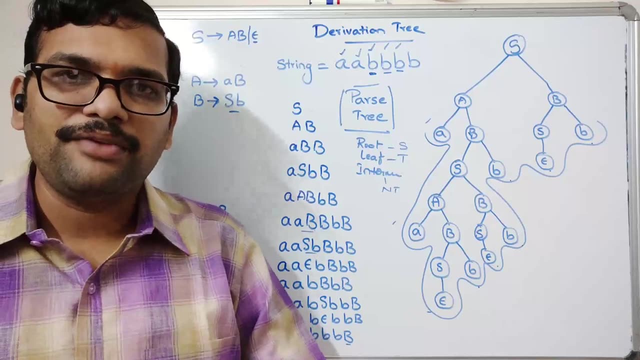 right, So hope you understood this derivation tree and the derivation tree. So let us stop here, and if you are having any doubts regarding this one, feel free to post your doubts in the comment section. Definitely, I will try to clarify all your doubts, If you.